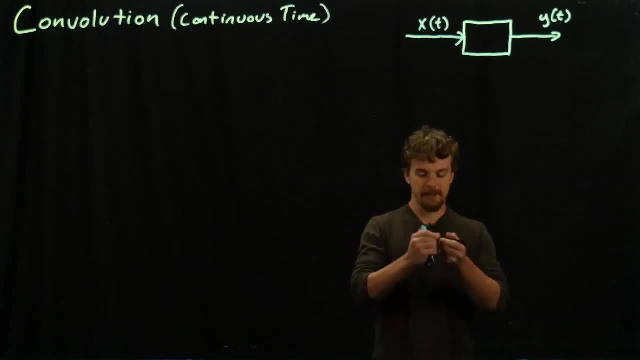 As we'll see, it gets to be some really long integrals involved and whatnot, but it's important. So the idea is that we have a system with an input and an output. I mean that's kind of the definition of a system. 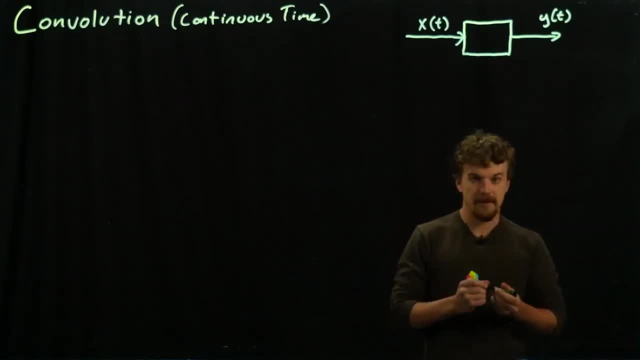 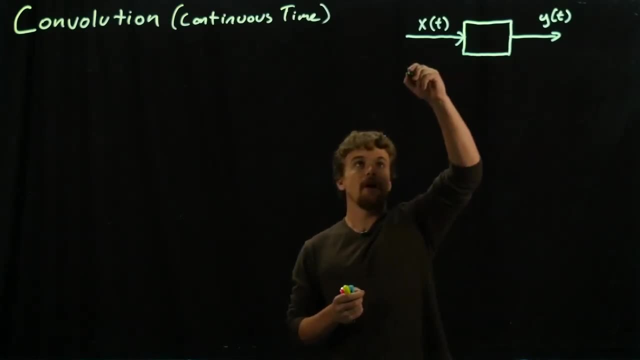 And let's say that we've done some experimentation or some good modeling. And let's say we know one thing about the system. Let's say we know what it outputs when we input as x of t, if our input is an impulse function, Now this impulse function is a theoretical function. 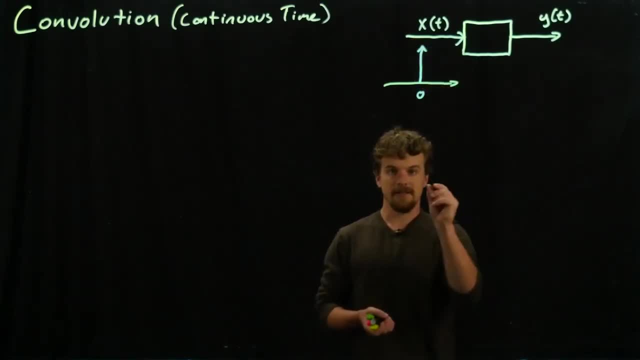 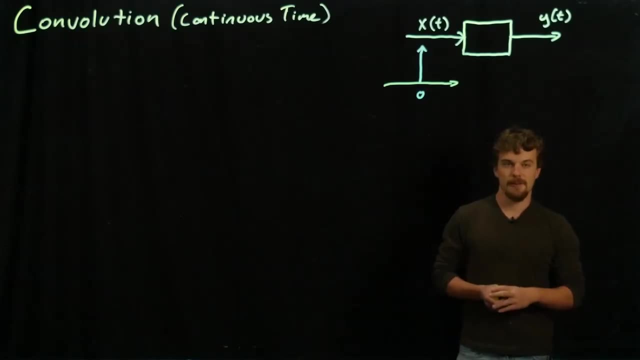 The idea is that it's infinitely tall, it's infinitesimally wide and when you integrate over it, it will integrate to 1.. So those are just some mathematical things, Those are just some mathematical properties we've come up for for this. 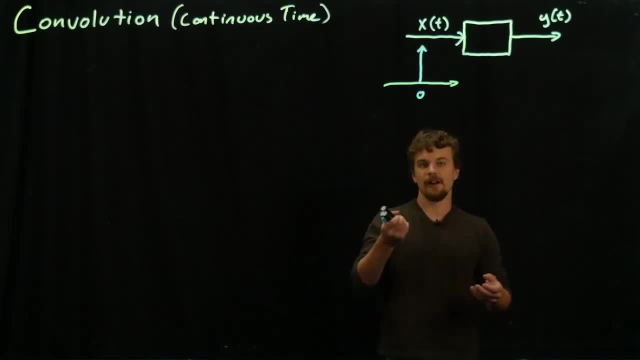 And, as we'll see, it helps us. It's theoretical, but it helps us do practical things. So let's say we know what the system outputs when we put this in, And let's say, in this case, that this system is going to output function. 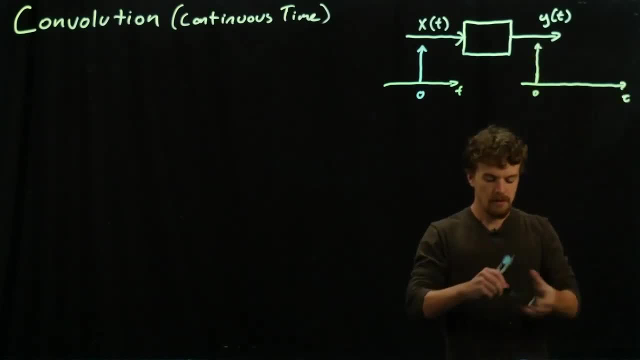 Let's say that this system outputs a function that can be modeled as: Okay. so this is what we'd call impulse response. We put in an impulse. this is the response we get for putting in an impulse, and it's usually denoted h of t. 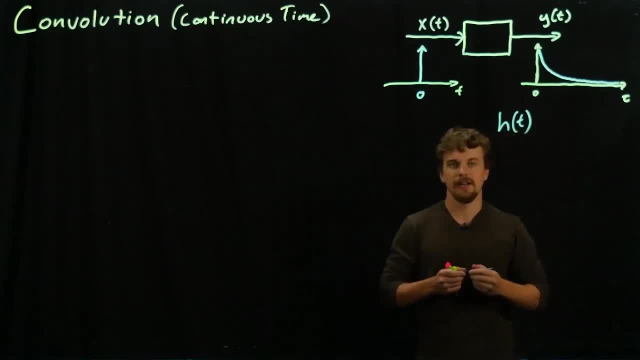 And I'm picking this arbitrarily. I'm saying: suppose this system outputs this for an impulse. Let's call this 2 times x of t, Let's call this 2 times e to the negative t. That's actually a practical impulse response we see from systems, from some systems. 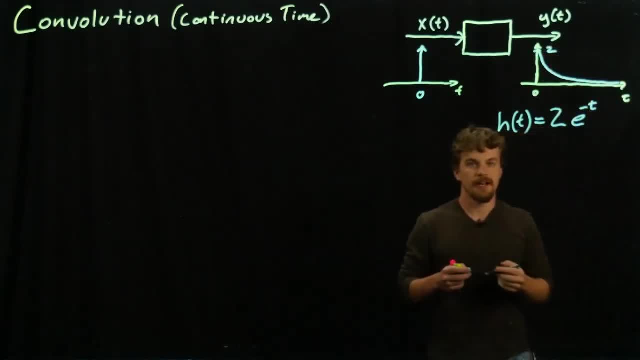 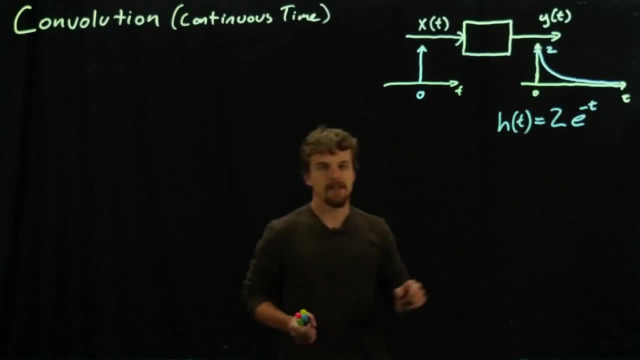 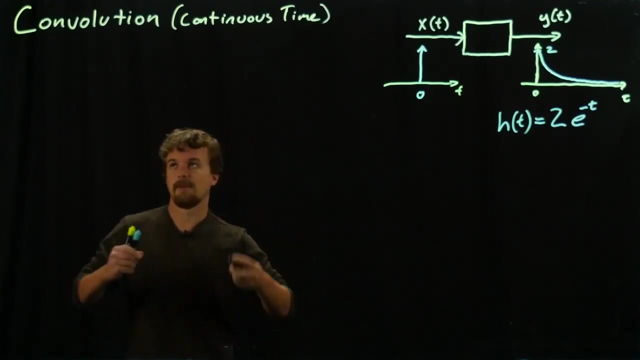 So this would start at 2 and exponentially die down. Okay, so, given that we know this, the idea of convolution is that we can take any input, xt and this impulse response, and we can get the output for any input. Let's say that our x of t. let's come up with an arbitrary x of t and see if we can do this. 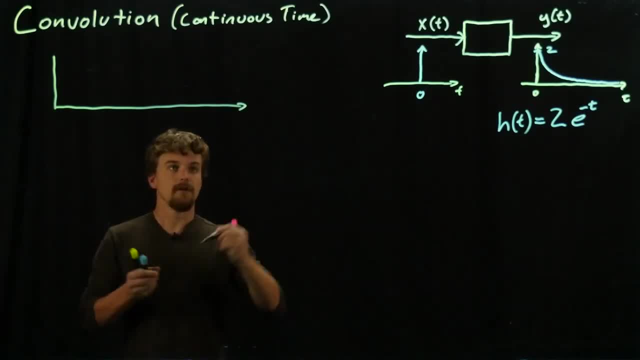 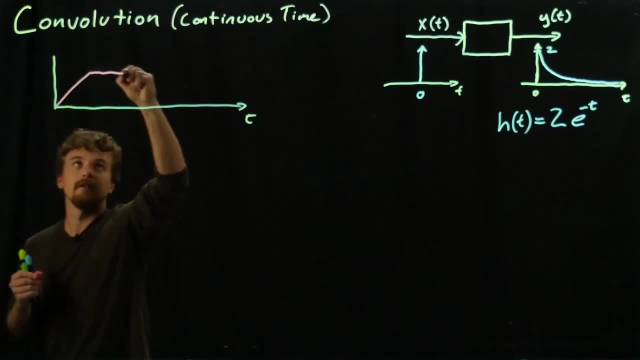 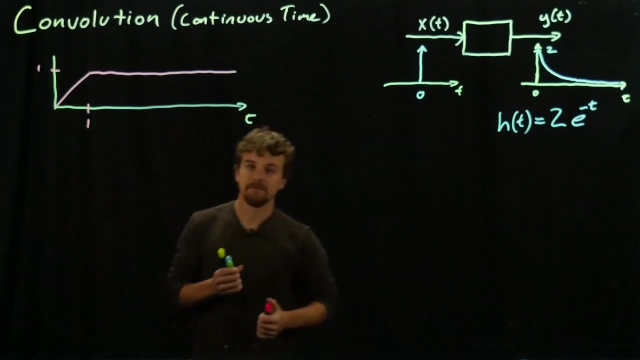 So let's say that for our input now we will give it a function that looks something like this: Let's say that this discontinuity here happens at t equals 1, and that goes up to a height of 1.. So we're going to have to describe x as a piecewise function eventually for doing the actual integration. 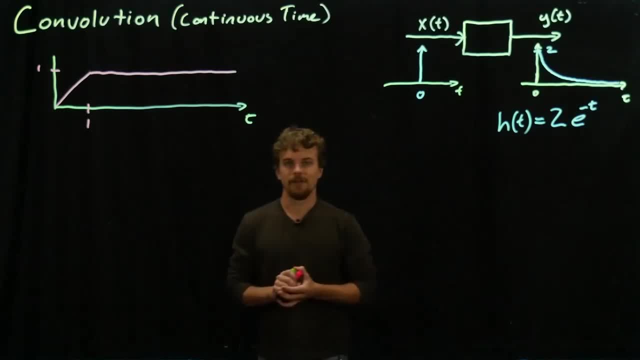 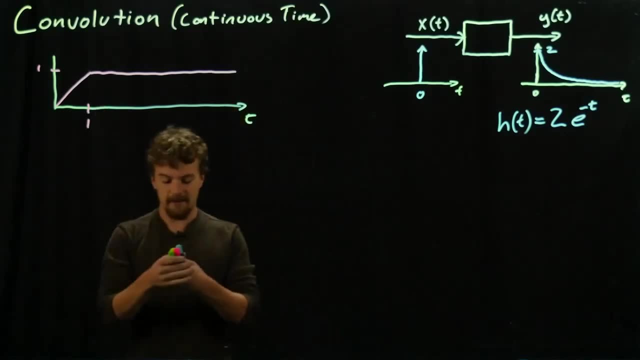 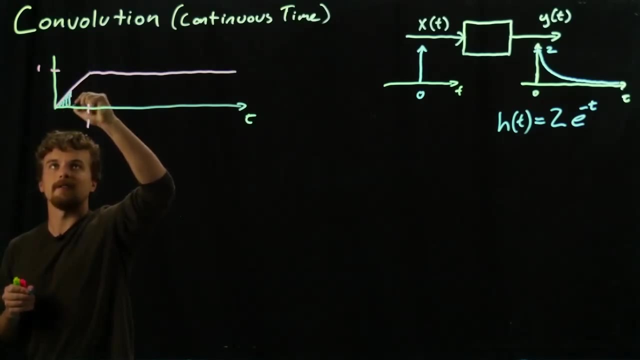 So what, conceptually, do we do here? What we do is we treat x, this input, as if it's a bunch of consecutive impulses. We say we theoretically break x up into infinitely many impulses, all scaled by the value of x, all the way across. 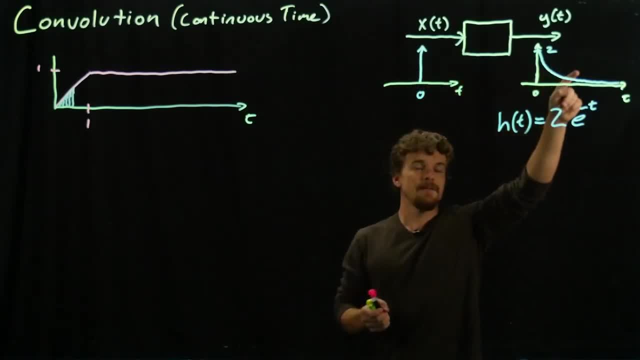 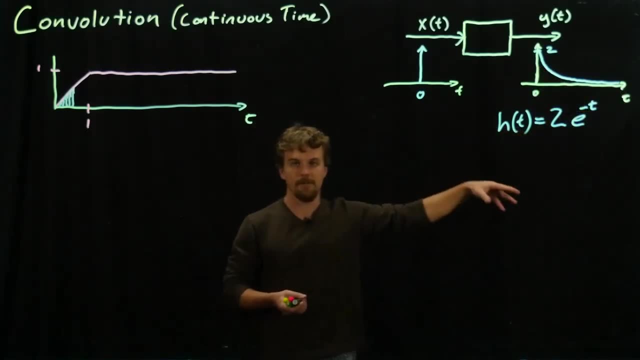 And we are shoving those impulses into this system and we'll get a combination of these impulse responses. If we put a bunch of impulses in, we're going to get a bunch of impulses responses out And they're going to be added together. 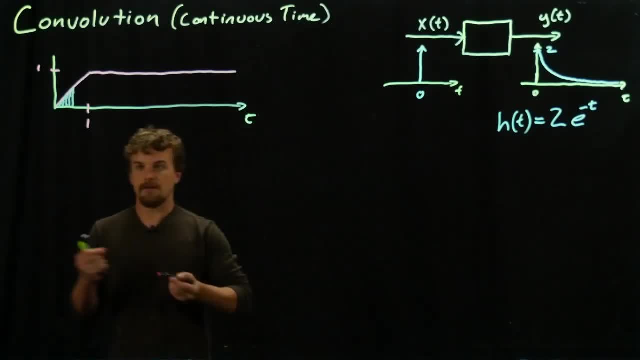 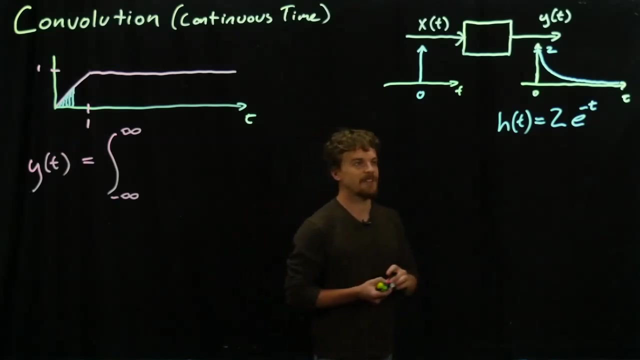 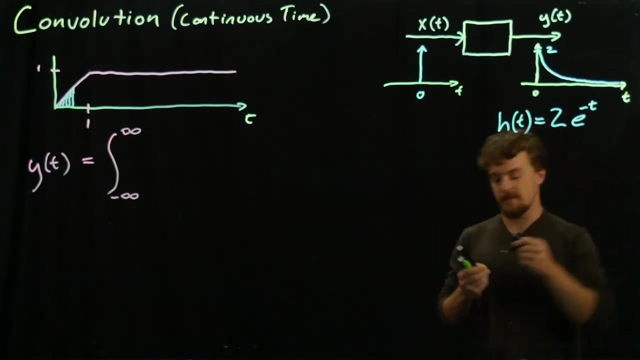 Without getting into the proof of it. what this results in is that our output here is going to equal the integral from negative infinity up to infinity of. Okay, so we're going to introduce a dummy variable, tau, We want toactually. I'll just write out the statement first. 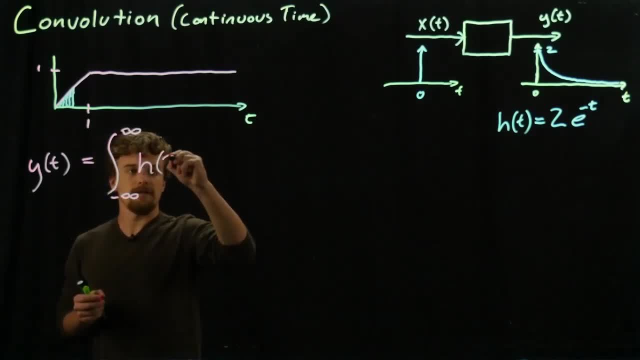 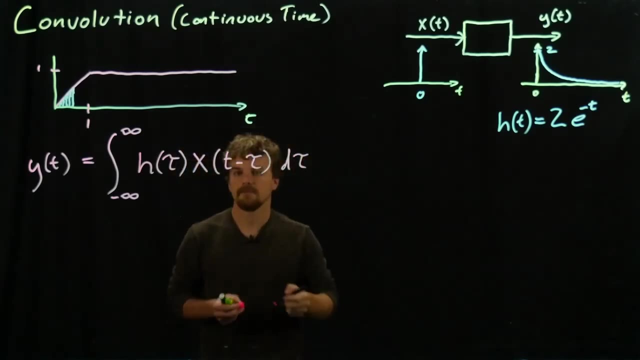 So this is going to be h of tau, our dummy variable. So this is going to be h of tau, our dummy variable, Times, x of our input of t minus tau, And we're going to integrate over tau. So it's a little bit hard to picture why we use this dummy variable. 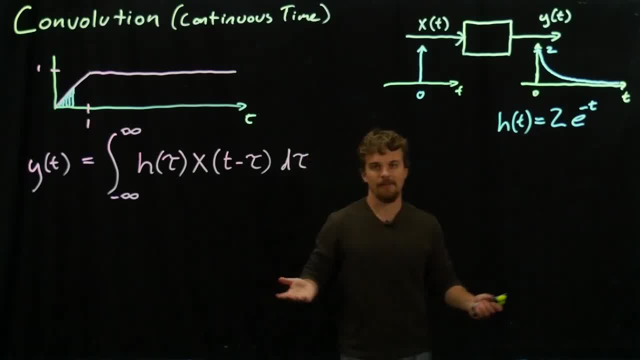 but the idea is that we're integrating over time to get a function in time, So we have to introducewe wouldn't want to call these both t, because we're only integrating over one of them. So just roll with that for a bit and we'll see how it works. 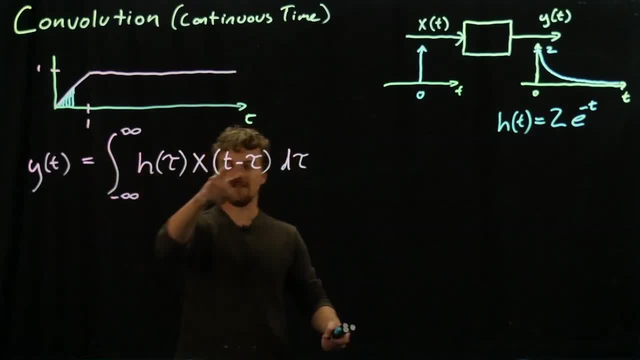 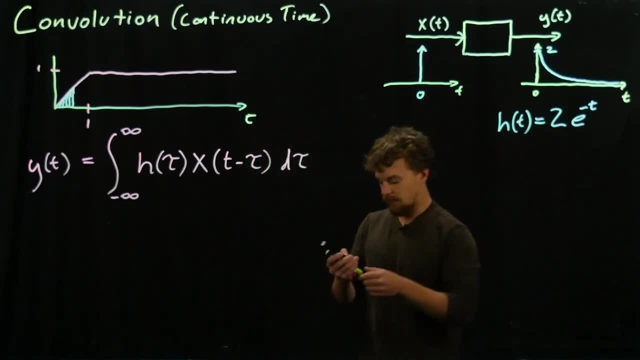 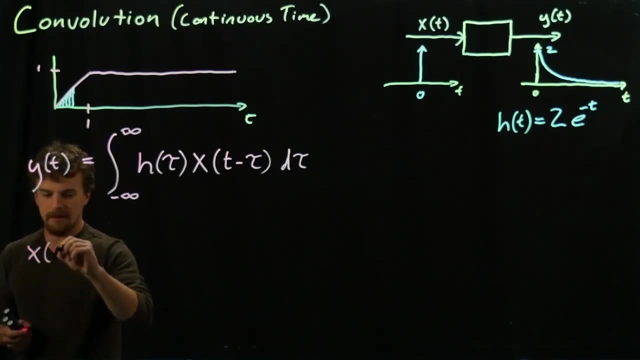 So this is going to give us our output y of t for any x of t that we can come up with. So let'sso we already defined h of t, Let's briefly define x of t explicitly. So we could say that x of twe arbitrarily came up with this. 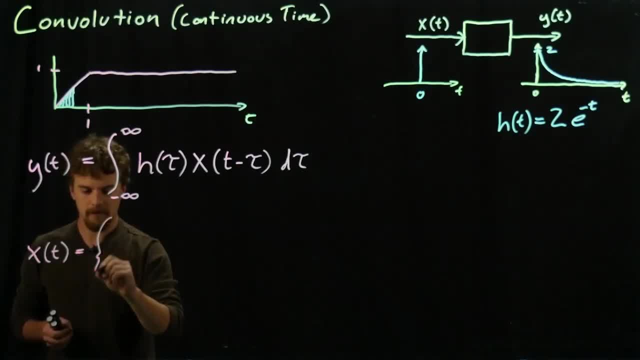 but we'll try to describe it as a function. So let's see Beforewe're going to go ahead and assume this: x of t starts at t equals 0, right, Like over here, we got nothing. So x of t is equal to 0 when t is less than 0.. 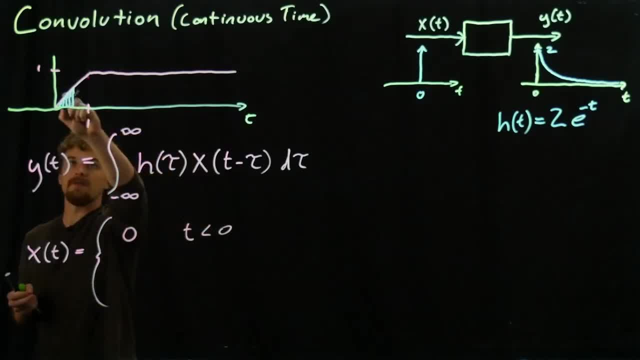 x of t is equal towell. what would this function be? It's just from 0 to 1.. That function would be just t, right? So we haveat any value t. the function is also equal to that value. 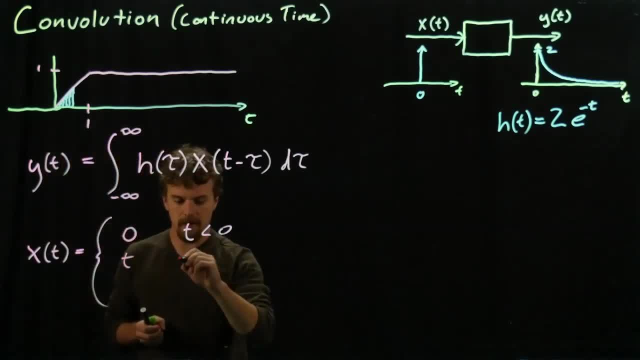 So x of t is equal to t for t greater than 0 and less than 1.. And then we see it just kind of levels out and we're going to assume this kind of just goes on for eternity. We see it's equal to 1 for t greater than 1.. 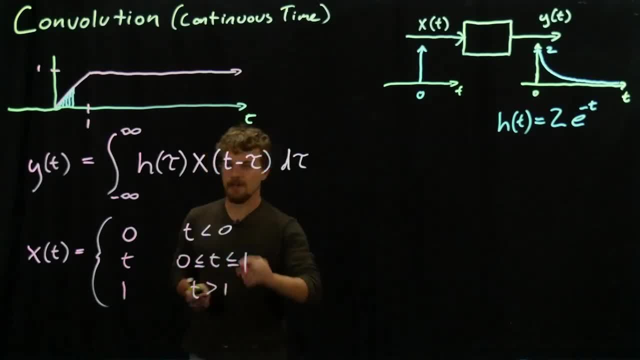 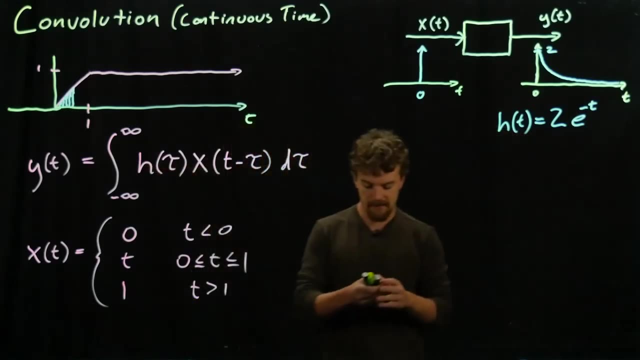 So we have to figure out how to do this integration operation here with this h of t and this x of t, And it's going to turn out that let's think about what this statement actually is kind of saying If we drew our dummy variable axis tau. 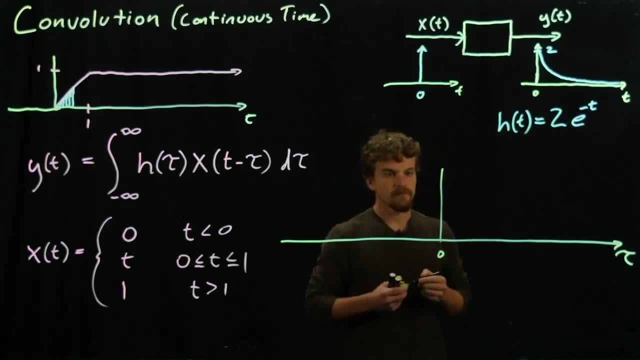 we'll pick a 0 point here Now. So h of tau is pretty straightforward, right hif, we just plug in tau for t, we'd get 2e to the negative tau. So we could graph that on our tau axis pretty easily. 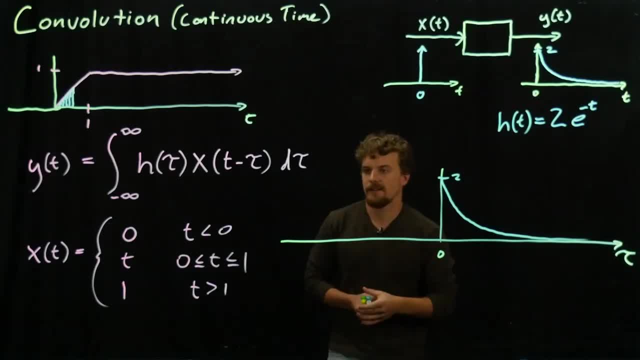 So that's our h of tau. And now what is x of t minus tau? We could think of this as a, So we could right shift by. So remember that this t is not a variable. in this case, We could right shift. 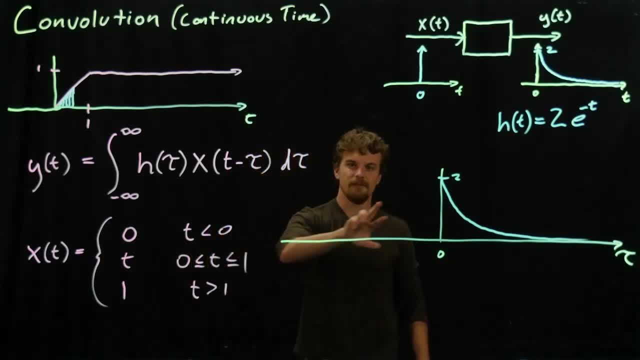 I'm sorry, left shift by this t And then it's of negative tau right. So we would mirror it around the y axis. We would flip it like that. So let's see what that looks like. So Weactually let's draw that in red. 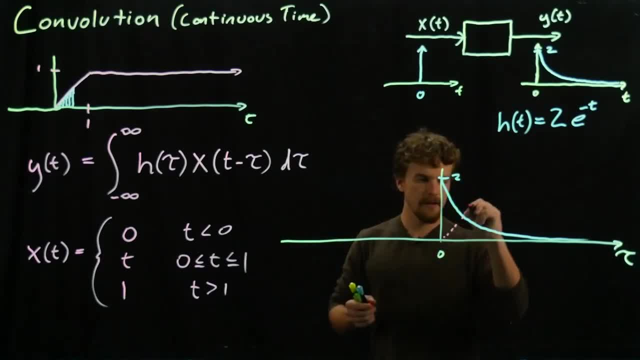 So our original x function looks something like that. Let's left shift by t and then mirror it, And what would that give us? It would give us something that looks like this: And then this original 0 point of our function is at t right. 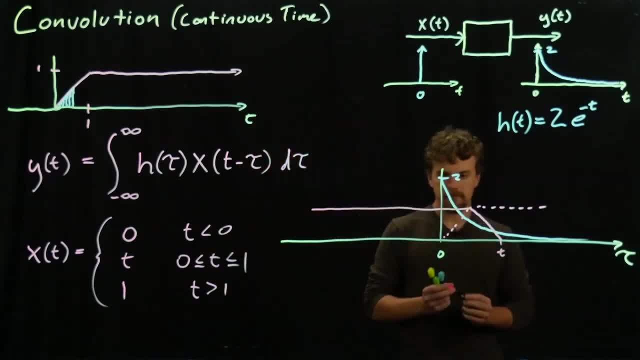 Is that more or less? Yeah, So we're going to have to erase the board here, But we're going to see that this integration, So we're taking the product of these two functions with x flipped like this, And we're going to do the integration. 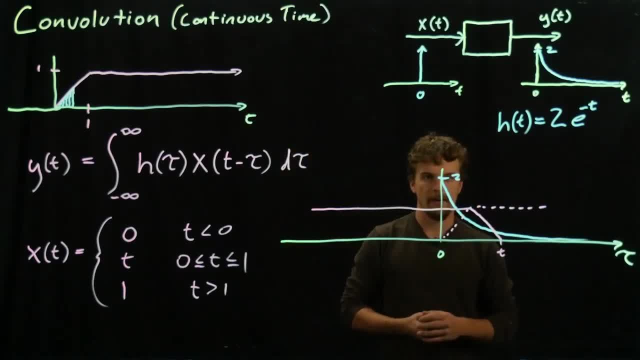 Since we have a piecewise function here, we're going to have a couple different regions where the integration is going to have different values, So we're going to erase the board a couple times here and do out the integration. But this is a good visualization of what's going on here. 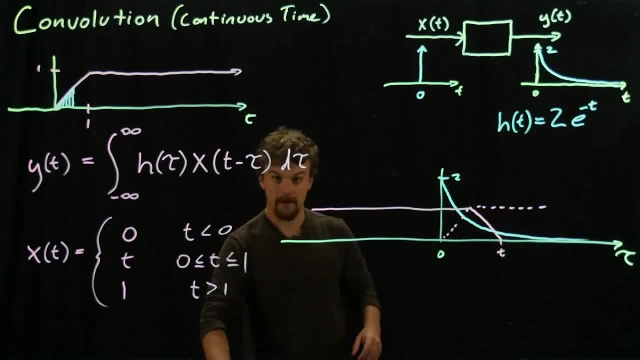 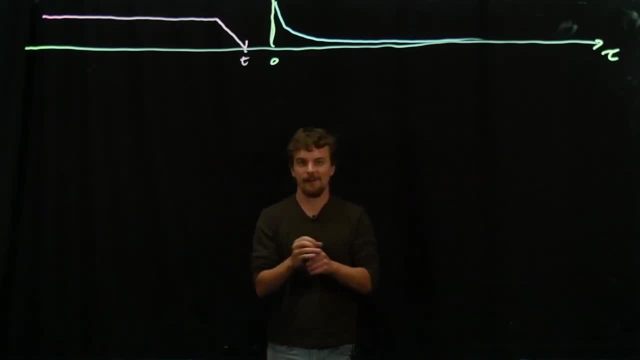 So we will deal with that right now. So now we have this dummy variable axis set up, with one of our functions just graphed normally and one of our functions shifted and mirrored around the vertical axis. So we're going to. There's a couple. 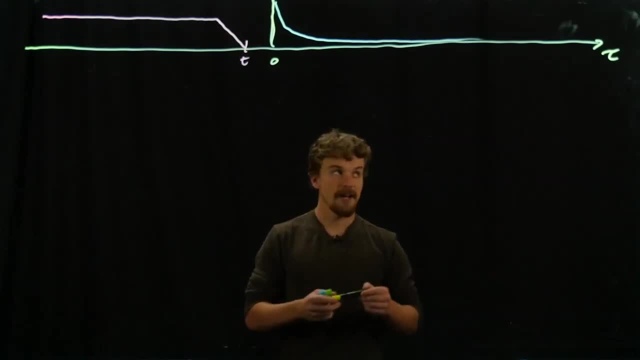 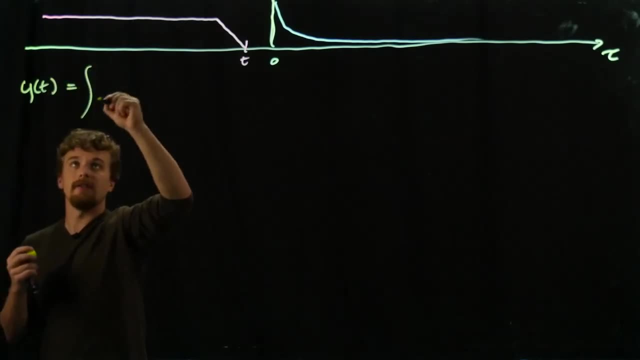 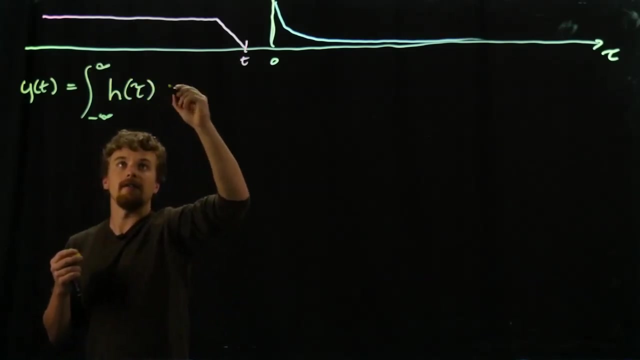 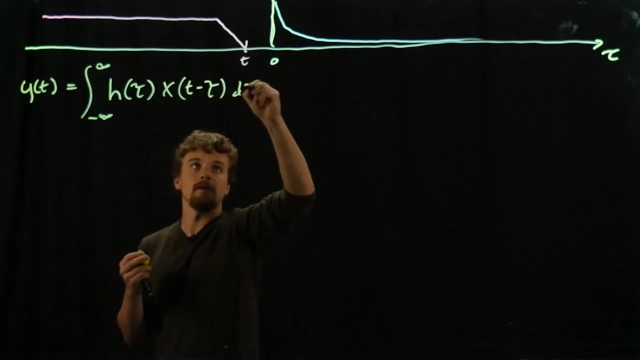 Okay, so remember what the convolution operation actually was. It was, We said y of t was equal to integral overall values of the product of our impulse response and our input shifted and flipped. So we can think of setting t, this t, to be different values. 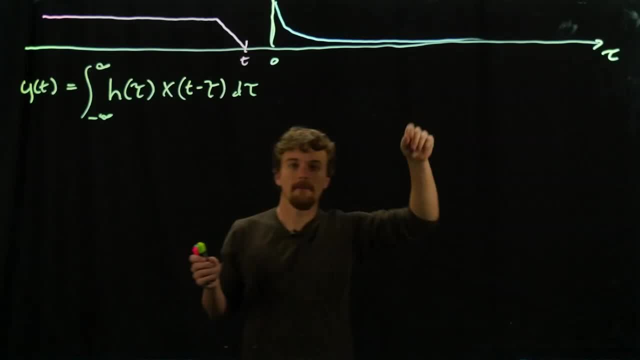 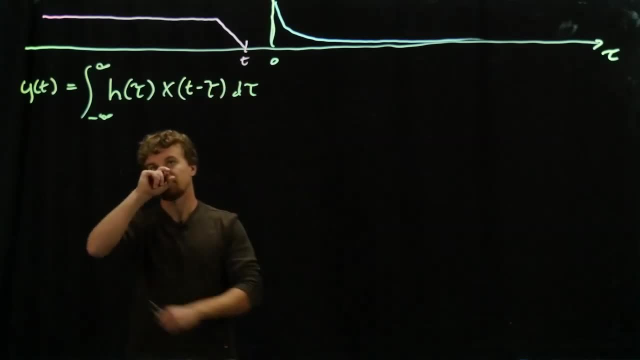 We're not integrating over it, so we can kind of just put it anywhere we want, And we can see that. So in this case we have 0 and t is less than 0 here, right? So what would happen to this expression when t is less than 0? 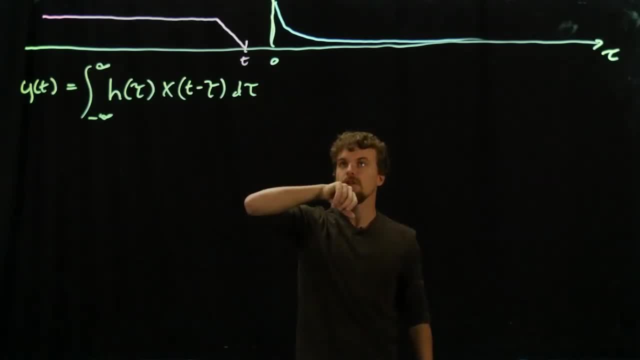 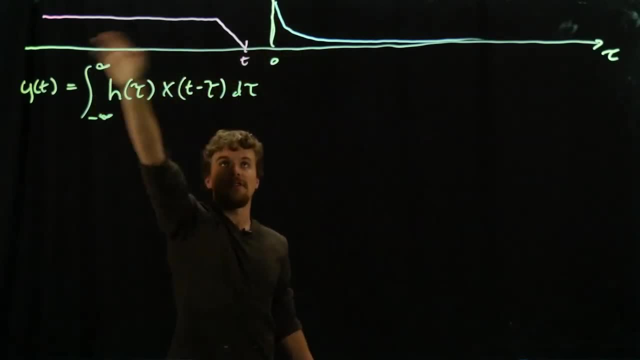 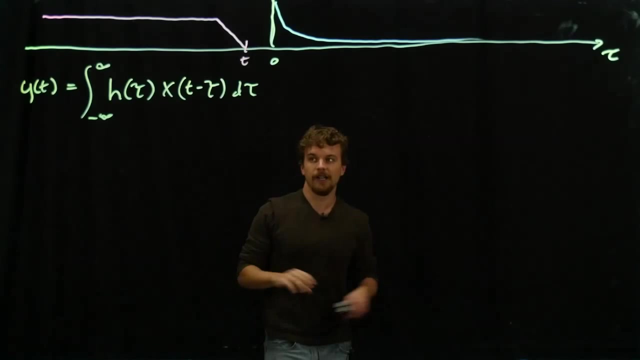 just from our graph of our situation here, We would see that their product, right, our impulse response is 0 over here and this function is Our input is 0 on this side, So the product of them is 0 everywhere, right. 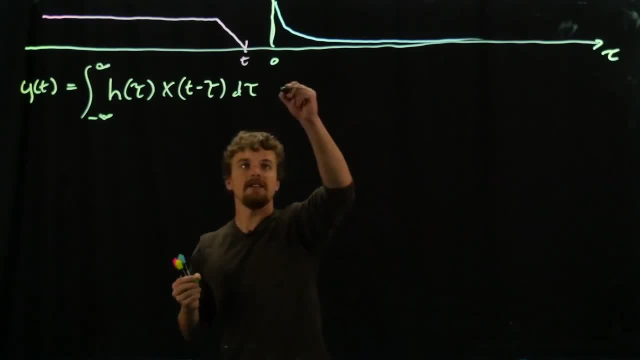 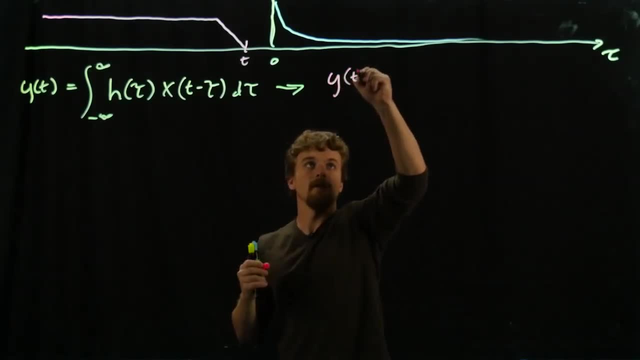 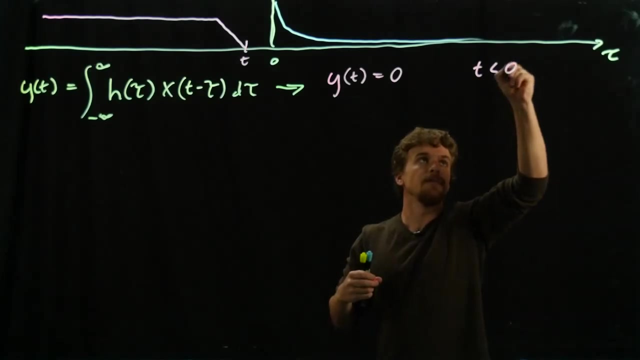 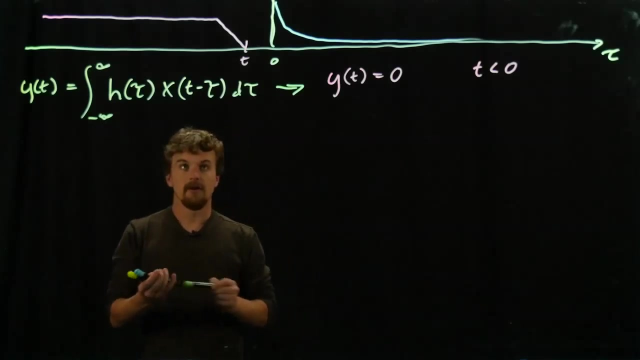 So in our first case here we kind of get the quick answer that y of t is equal to 0 any time t is less than 0.. For t: less than 0.. Okay, so that's one part of our integration. Now let's imagine that we shift t a little bit. 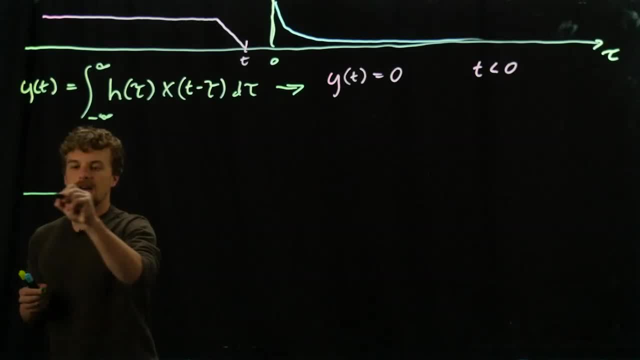 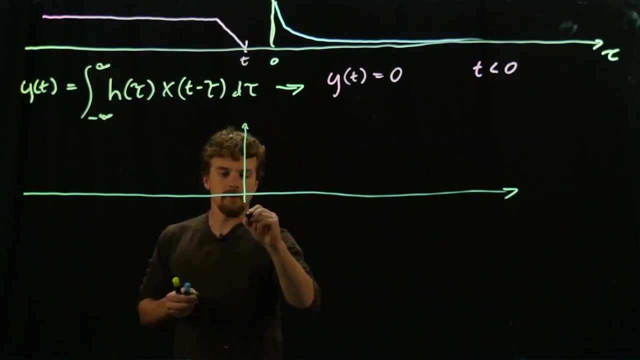 Let's make it. I'll redraw it here. Yeah, that one is much better So. So this is our 0 point. We will have our impulse response still graphed normally, And let's shift t so that it's just a little bit bigger than 0.. 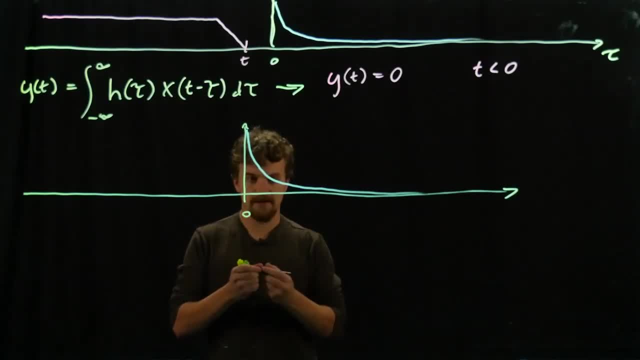 Let's say that we shift t so that it is in between 1 and 0. Actually, let's mark 1. As well. Let's say 1 would be around there, 1. Now we're going to put t somewhere in here. 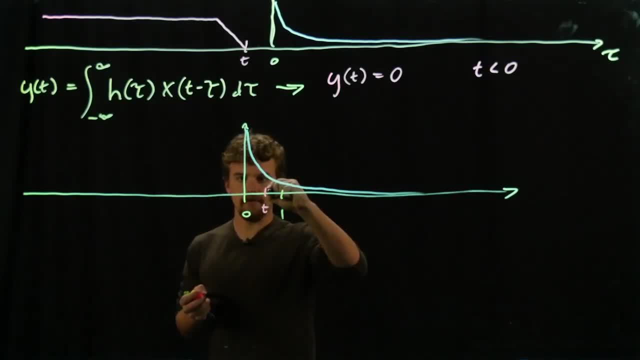 t, And now our shifted function would look something like this: Okay, so the reason we limited t in between 0 and 1 here is because we can see, as if we slide t up to 1, we would get our function fitting just perfectly in here like that. 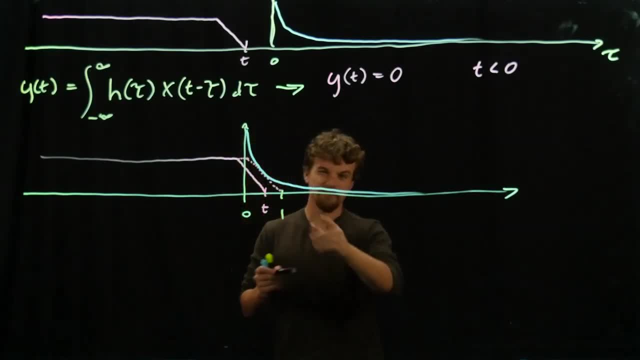 And the discontinuity would be at 0. And then we'll see that when t is greater than 1, then our integration becomes a little bit different. But let's do the integration for this where t is in between 0 and 1.. 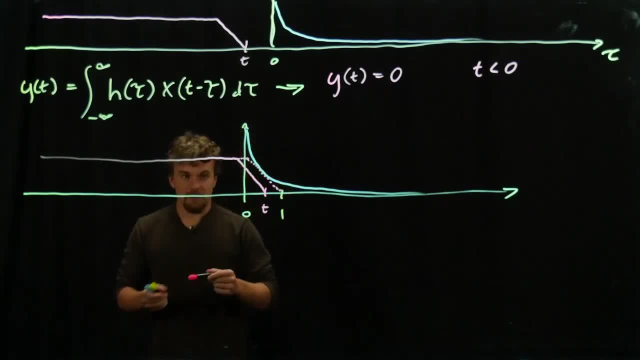 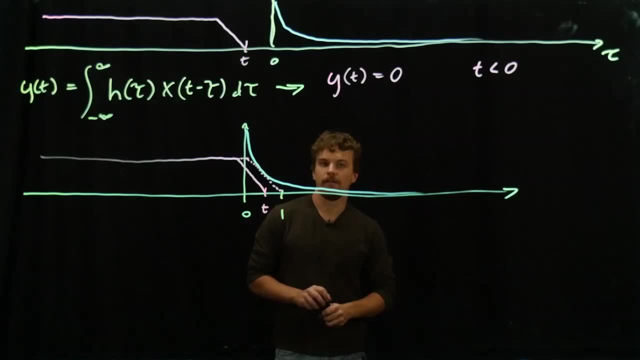 So we have to integrate the product of these functions right From negative infinity to infinity. Now again over here, the product is still 0, right. And then also we'll see our flipped function: here is 0 after t, right. 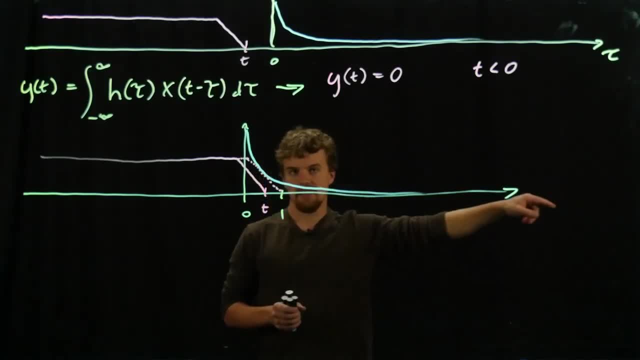 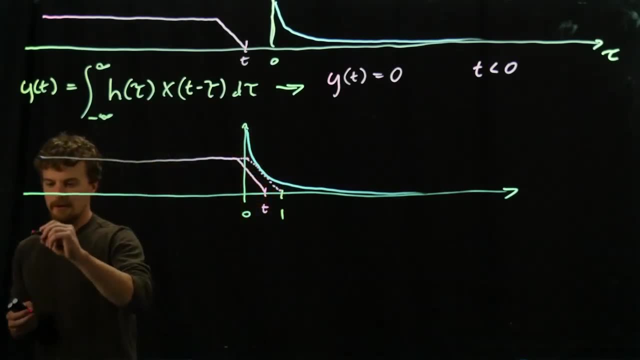 So for t, for any tau greater than t, the product of these functions is also 0. So the integration only has to be done. So we'll say for t actually yeah, for t greater than 0 and less than 1,. 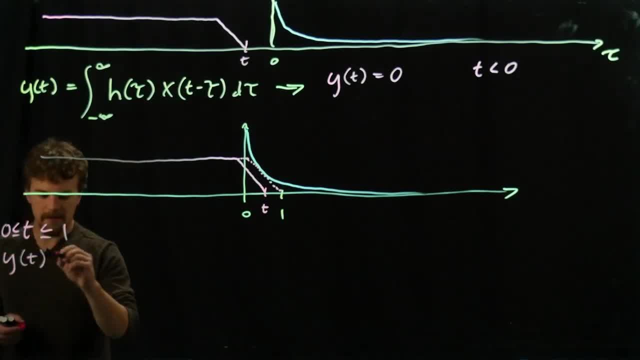 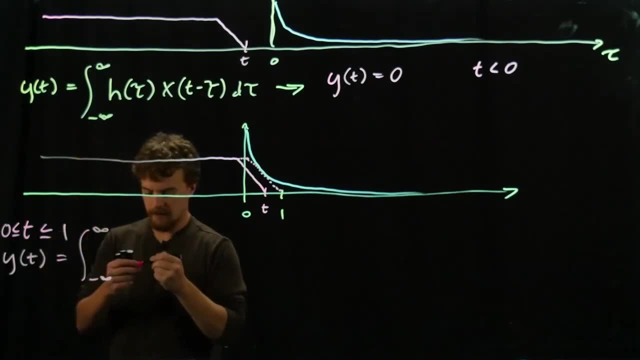 our y of t is going to equal the integration from well we'll start with negative infinity to infinity of so well we can do. h of tau is 2 times e to the negative tau, And then we're going to multiply that by our shifted and. 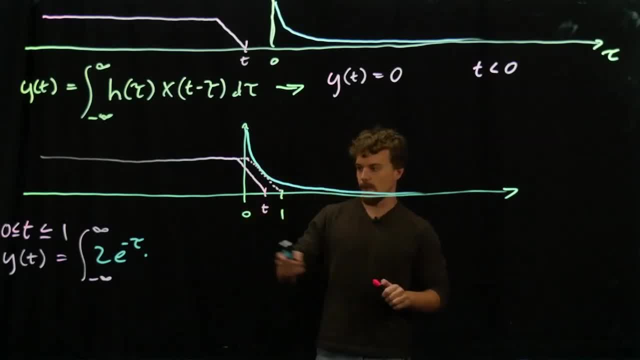 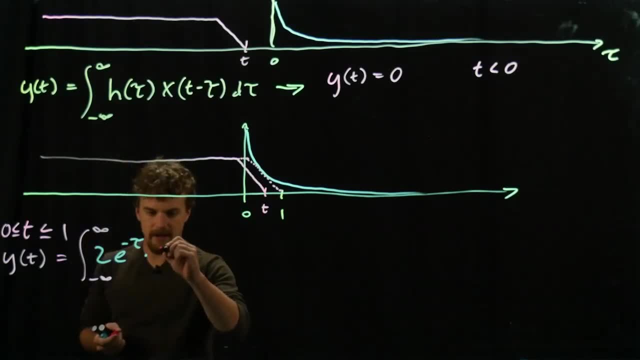 so what was so what? oh, remember what was x of t for t in between 0 and 1? It was just t, right? So for so now, x of t minus tau is just going to be t minus tau. 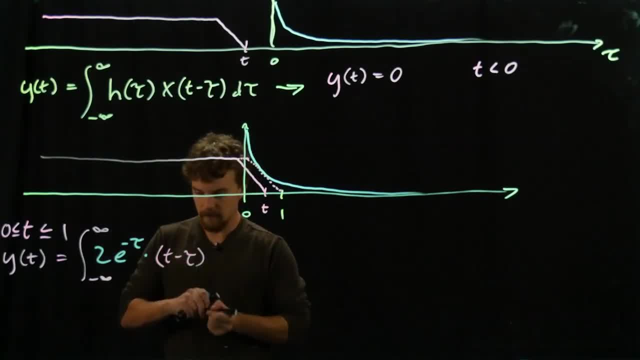 And then we're integrating over our dummy variable tau, right? Okay, so I could do the integration now. I did it on a piece of paper earlier. It's good practice, So actually I'll expand it a little bit just to make it a little bit easier for you. 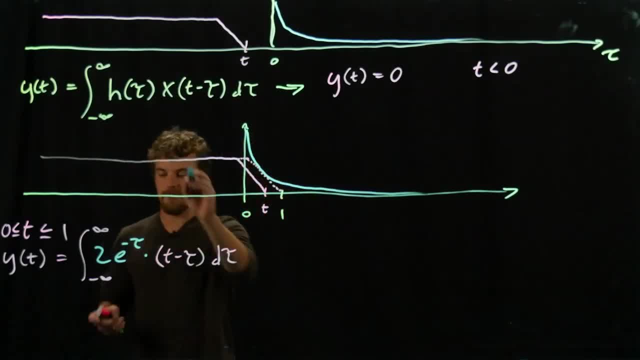 So remember what we talked about. We can change these limits. We don't have to do from negative infinity to infinity. We really it only has. in here. we only have a nonzero value between 0 and t, So we can simplify this a little bit. 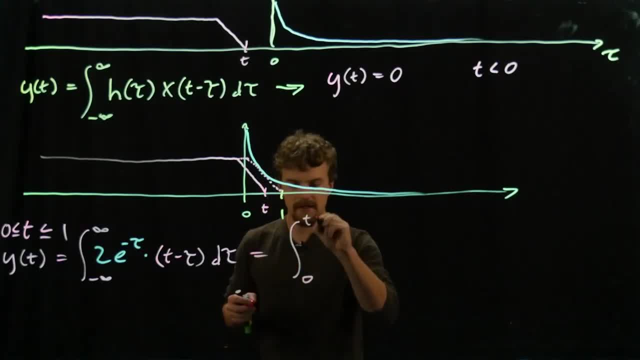 We can say: this is the integral between 0 and t of this expression. We can actually move: yeah, yeah, Yeah, let's move the 2 out here. So then we have e to the negative tau times t minus tau t tau. 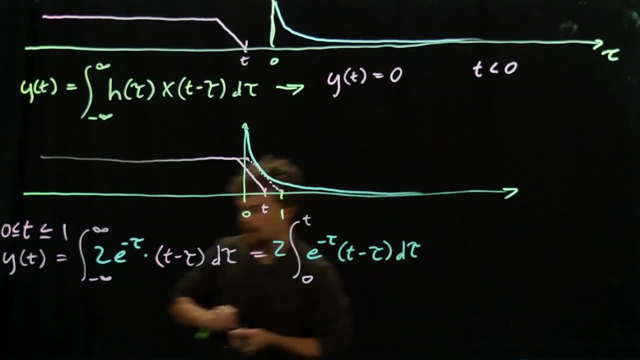 And yeah, we could expand that one more time. I guess You get that this is the integral. Well, this is 2 times the integral from 0 to t of. actually. yeah, it would be negative tau e to the negative tau t tau. 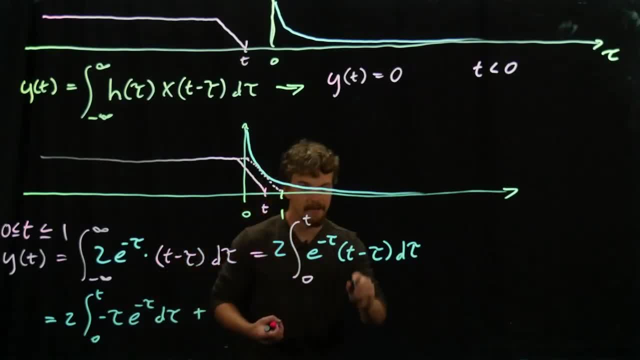 We're splitting our integration up into two separate terms. now, right, because we'd have to distribute this e to the negative tau to both places in there. And then this is plus 2t, integral from 0 to t of e to the negative tau, right? 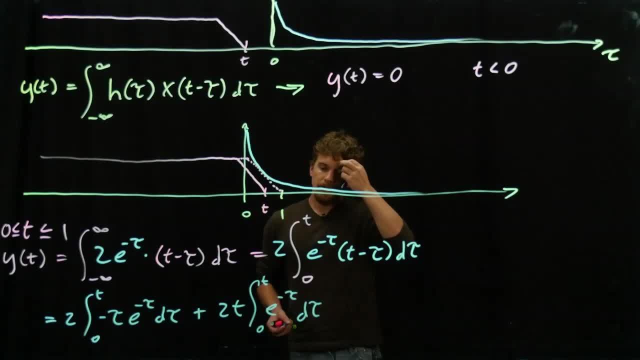 Now. so I'm not going to do any further integration here. I'm going to expect that you can do the work out And actually, if you have time, take the time to do it out and check my answer here. What I have for an answer for this part is equal to: 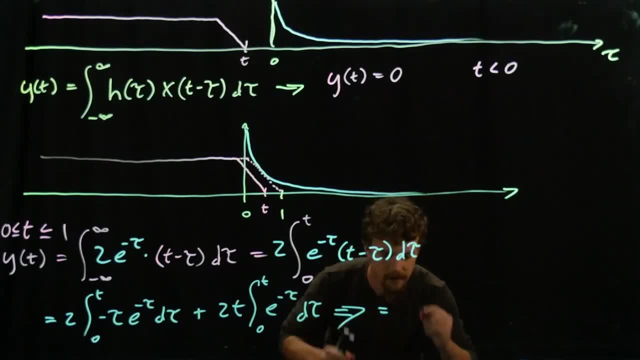 actually, let's write it in different colors. our final function here. So I have 2 times e to the negative tau plus t minus 1. And this is our output for our restricted input here. Remember we restricted the time domain here. 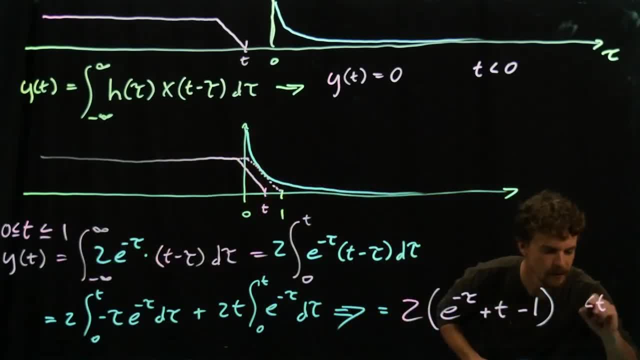 So this is our output for t greater than 0 and less than 1.. OK, so take a mental picture or an actual picture of this, because we're going to erase one more time and we're going to do the final step, for when we drag this t value past 1.. 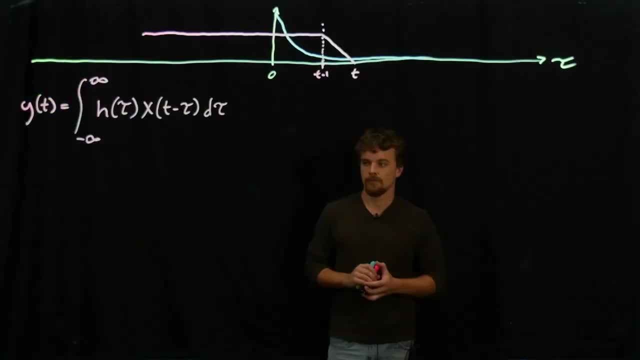 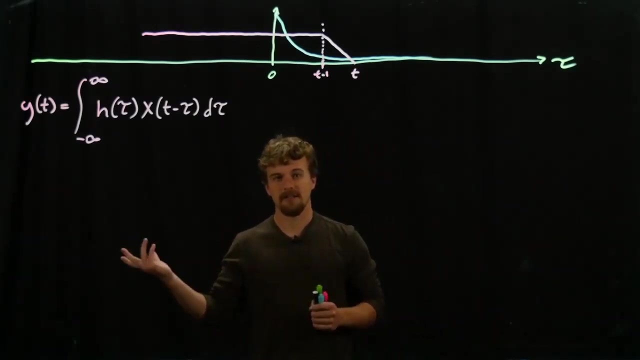 We're going to have to. we'll see what happens there. OK, we're back. Here is our final case for our convolution. So previously, up till now, we've restricted t to be less than 0.. We found our output was 0.. 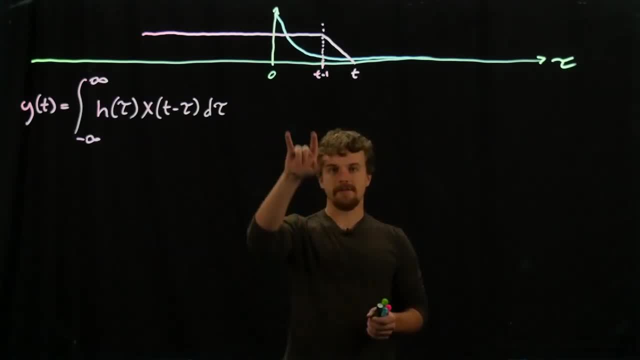 We found our output was 0 for that. And then we found what our function was for t in between 0 and 1.. And now? so now the remaining values of t are from 1 up to infinity right, So we're going to figure out what our convolution becomes for that. 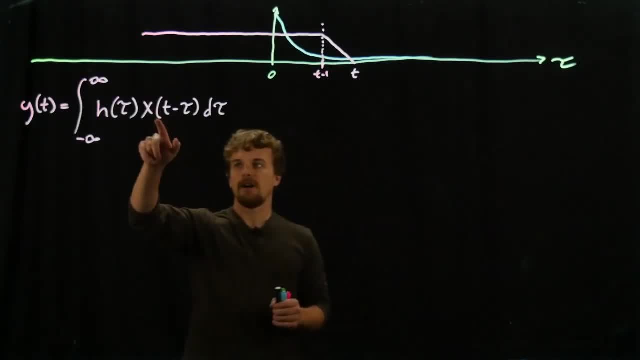 So we have to do this operation here. We've already so this pink function. here is our x of t and it's already shifted by t and flipped in this picture here. So we have to do the integration from negative infinity to infinity of the product of the two things we see right here. 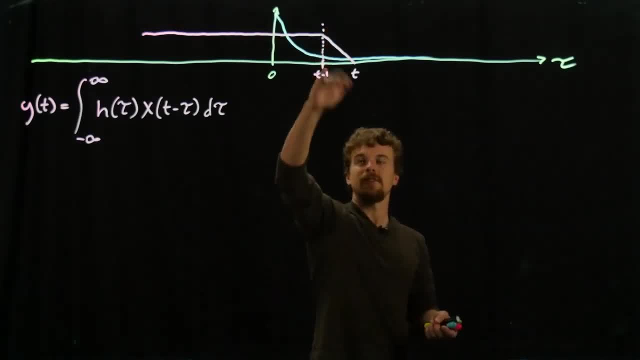 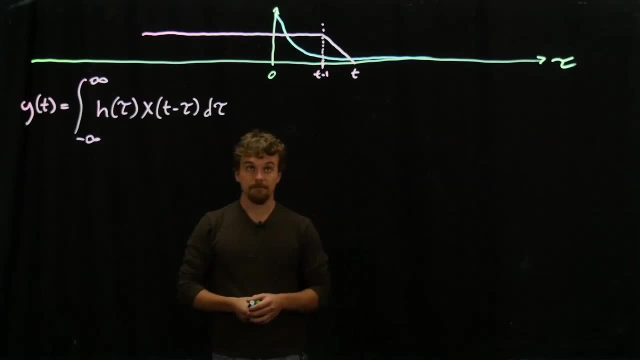 So we have a little discontinuity here, So we're going to have to kind of break our integration up into two parts. So let's first say that well, let's integrate the first region here. Our x function is continuous from here to there. 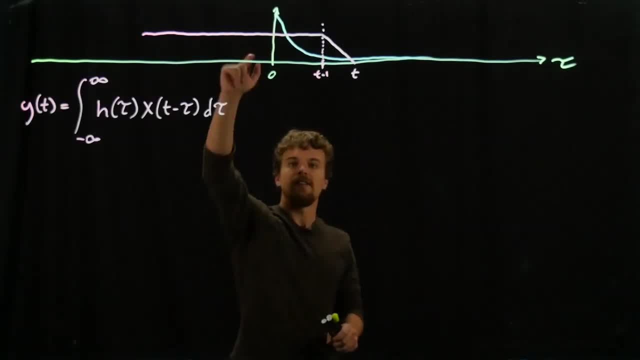 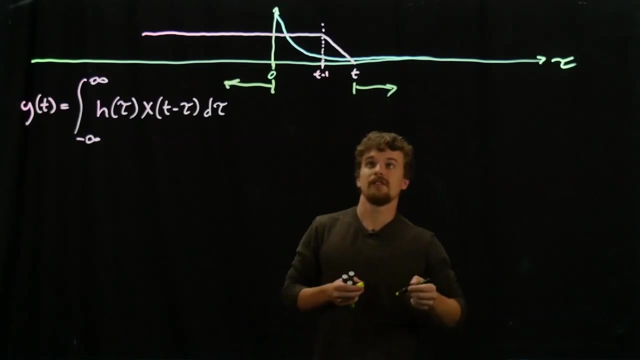 What is that? Well, yeah, so again, our product of these two things are going to be 0 outside these regions, right. Anywhere from that way from 0 and anywhere that way from t. right, The product is all going to be 0.. 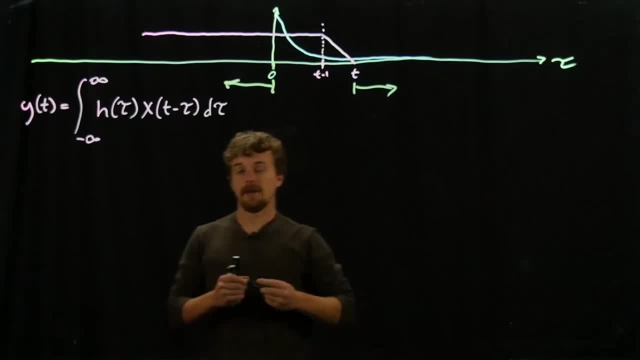 So we only have to do our integration from here to there. So how do we set that up? This is going to be so. let's first do the integration from 0, and remember, we can use this t value. We're integrating tau, so we can use this t value as a limit for integration, right? 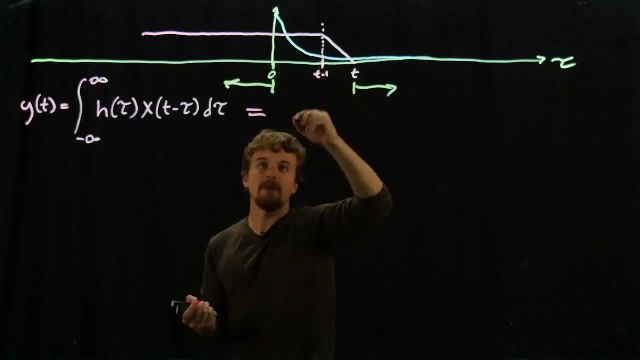 Let's do the integration from 0 to t minus 1 of this. So that would give us now what are our functions here? Our blue function here is still just 2.. 2 times e to the negative tau. And now what is our x of t for this region? 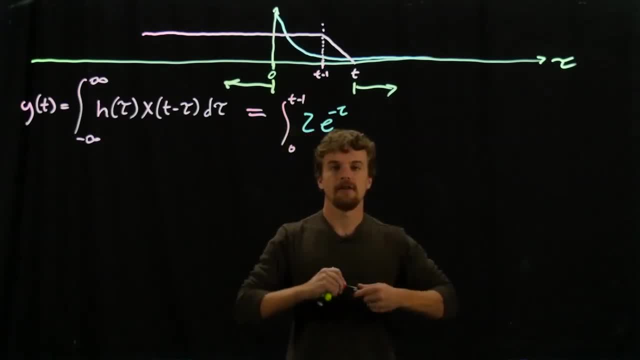 It's constant, It's just 1, right, So x of t minus tau doesn't really matter, It's just 1.. It's just a constant. And then, yep, then we're integrating this over tau. And what do we get? 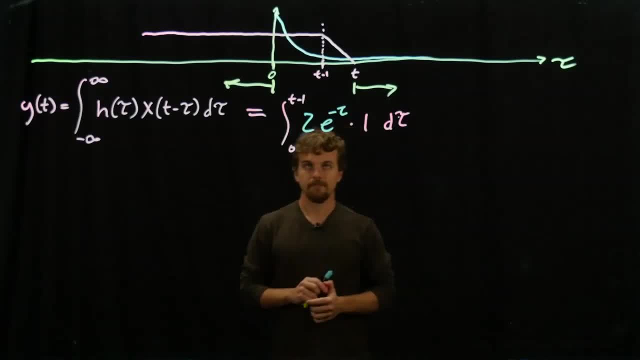 Actually okay. so let's just set up the rest of the integration too. We also have to integrate this little region here. So we're going to add to that integration, to this integration. We're going to say: this is the integral. 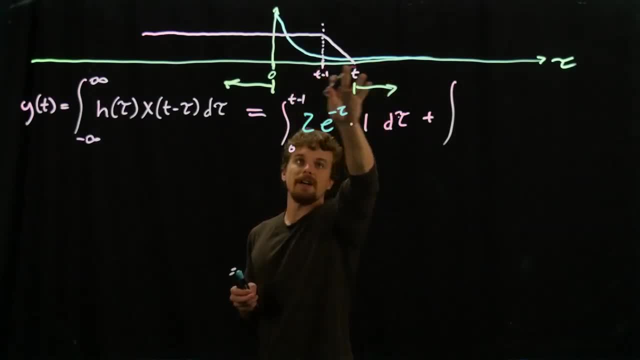 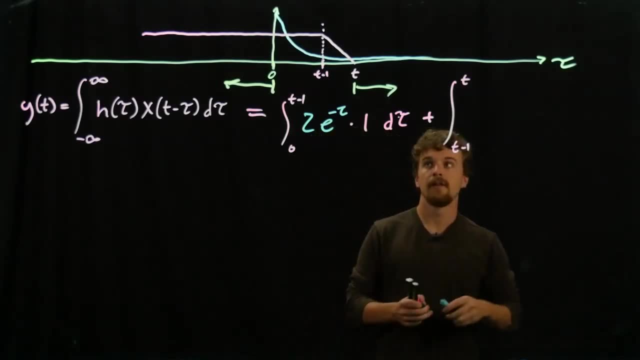 Now, what are the limits for this integration? We would go from t minus 1 to t right Of the product of our. again, our impulse response is still 2.. e to the negative tau. And now our flip, our t. 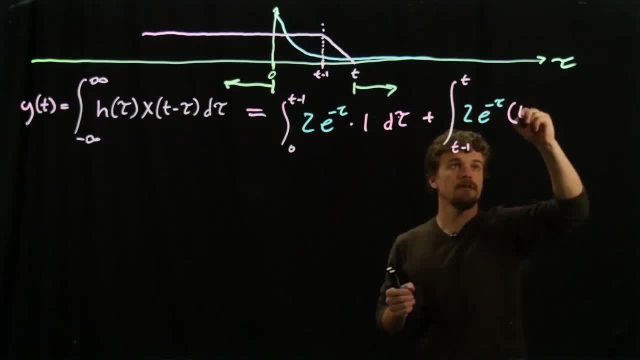 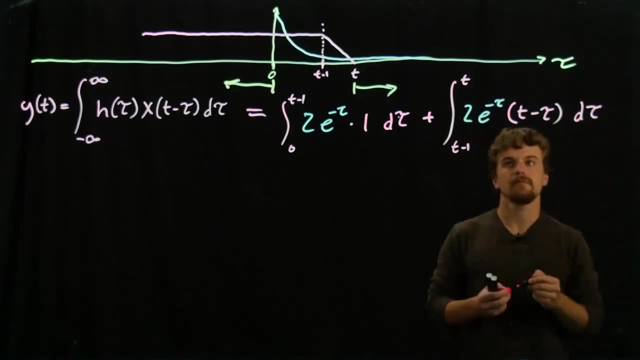 x of t minus tau is just again t minus tau for that, And then again we're integrating this over tau. So now, so this sum here gives us: this part is this region, This part is this region, And then, like we talked about, the rest is going to be 0. 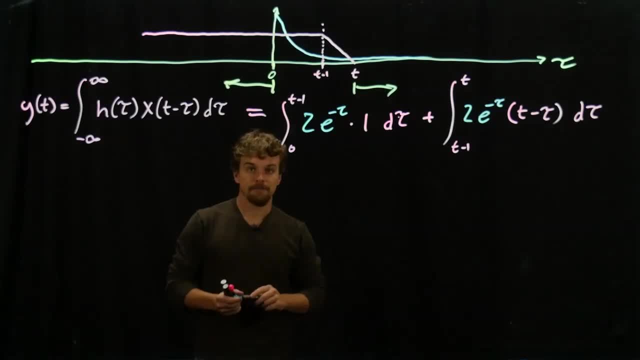 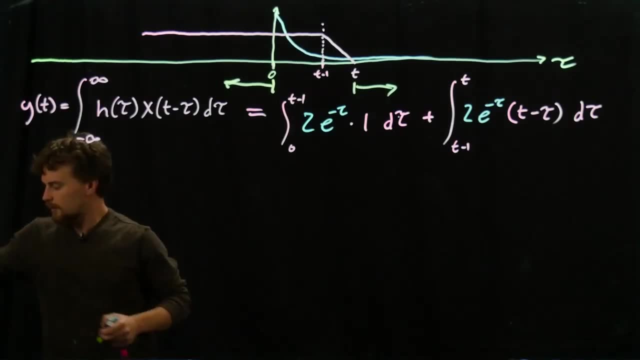 So we'll expand this out a little bit. We can keep this, I believe. let me look at my notes here for a minute. So we can expand this all out: equaling 2 times integral from 0 to t, of e to the negative tau. 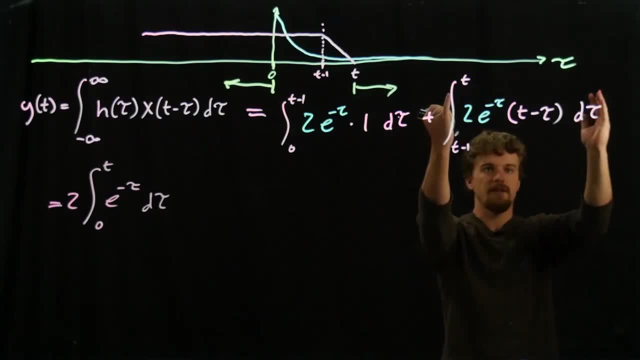 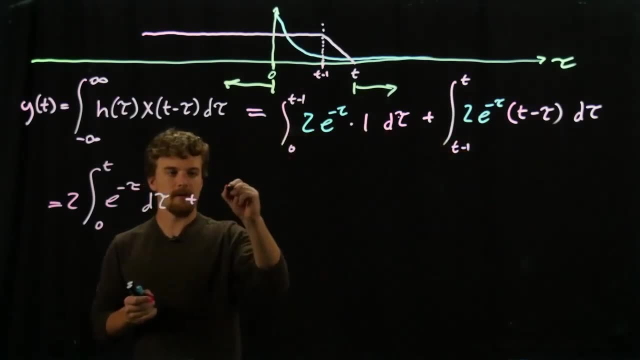 And again we have to split this part up into two different integrations. right, Because we have to distribute that in. This would become plus. we'll distribute this in, it'll be 2t times integral. Remember t is constant. 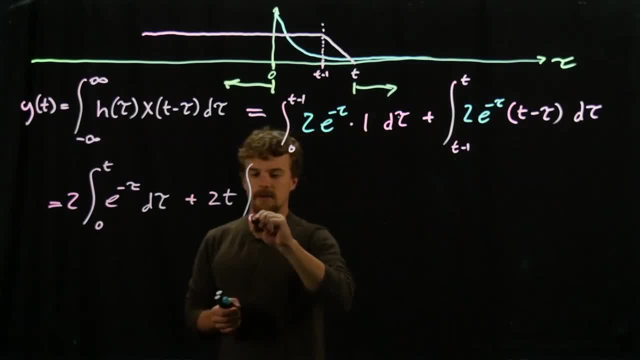 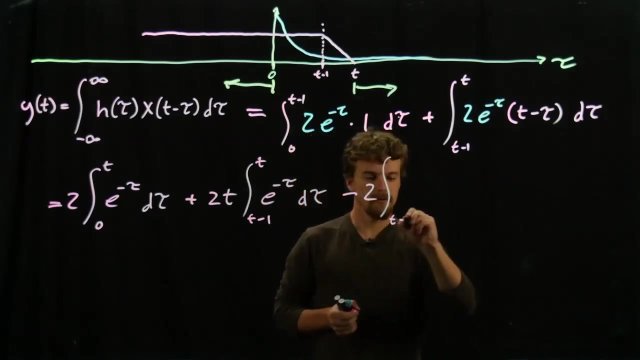 so we can just pull it out of the integration. We're going to go from t minus 1 to t of e, to the negative tau, right t, tau, And then our final term would be, from distributing this to the tau, This would be equal to minus 2 integral from t minus 1. 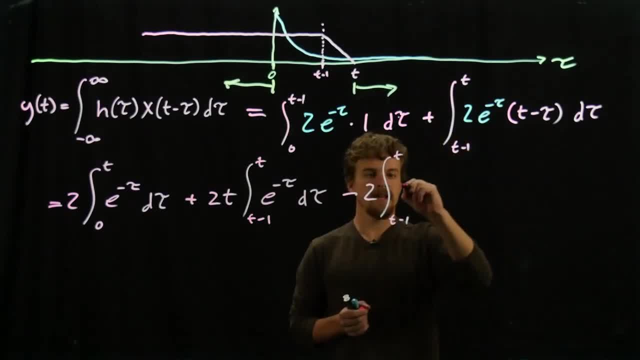 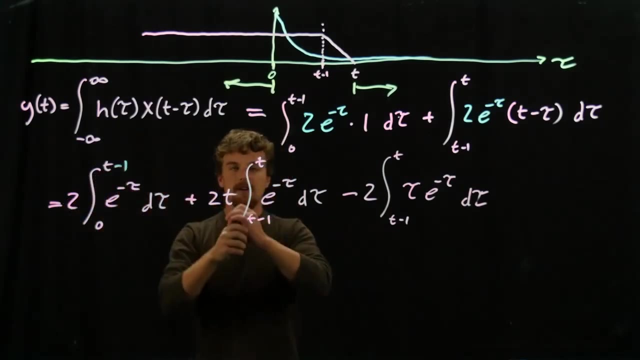 t of tau e to the negative tau, t, tau. Are you sure, Yep, yep, Okay. so previously, when I defined this little region here, I said it was 0 to t. It is from here This part of the integration. 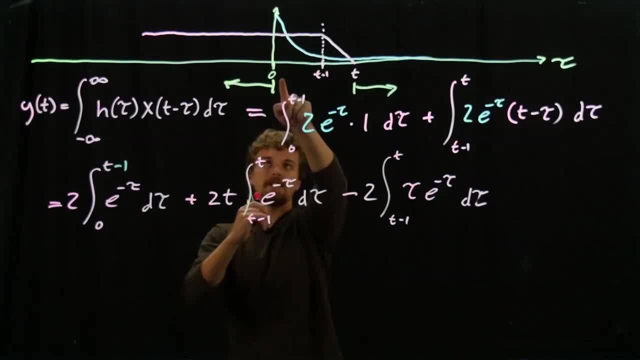 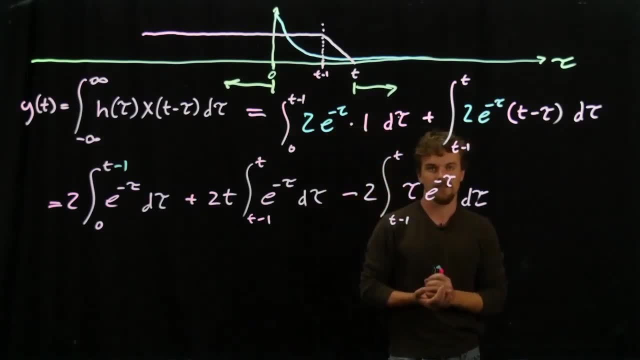 Okay, so I put it in up here and just failed later. So this integration is this region from just from 0 to where our x function becomes, where the discontinuity in our x function is Because there's no way to integrate over this. 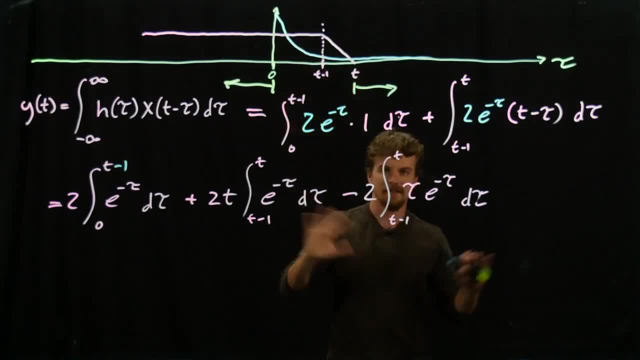 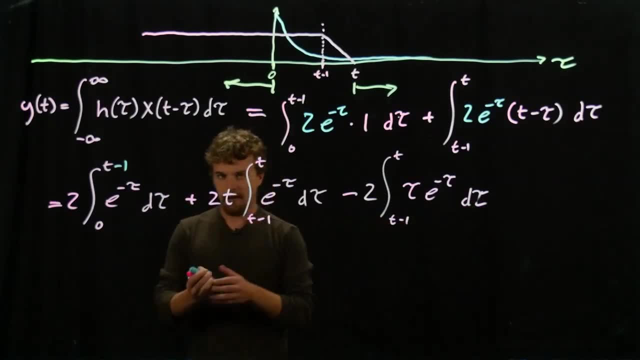 There's no way to describe this function all the way from here, all the way to t, as a continuous function. We have to do it piecewise. So this I'm going to. I mean it was a lot of work doing this integration out here. 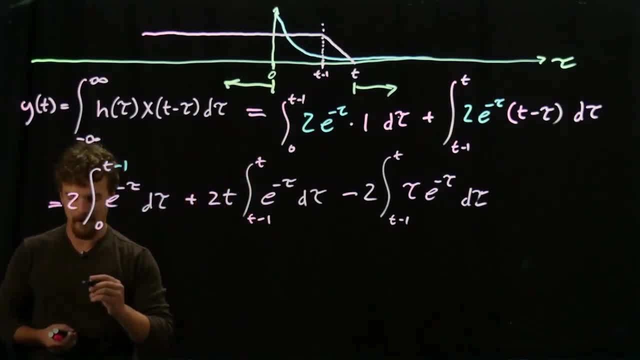 So I'm going to expect that you can do that and maybe again cross-check my answer Now. the result I got here- everything here- is equal to 2 times e to the negative tau. e to the negative t my bad. 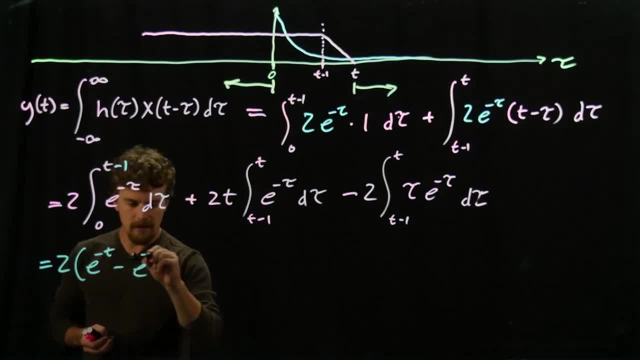 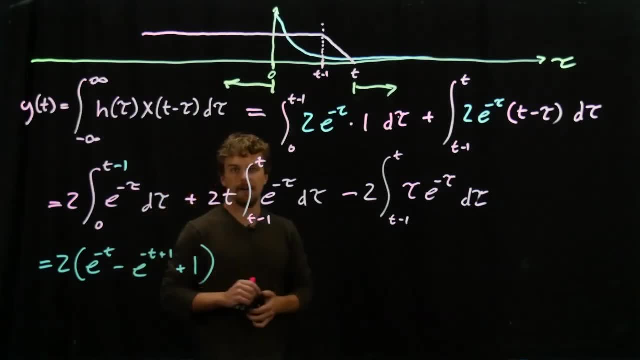 plus minus e, to the negative t plus 1, plus 1.. So remember our restrictions on our t or the value of t. now, This is for any t that's greater than 1, right, For t greater than 1..